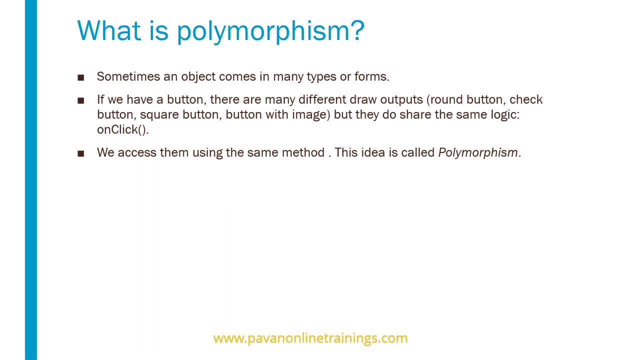 So if you have a button, so there are many different route woods, like a round button, check button, square button Or button with some image, but they do share the same logic. So whenever we click on the button it will do the same thing and 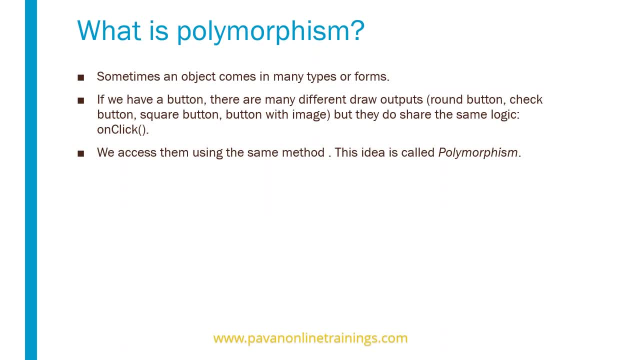 We can access them using the same method. So this idea is basically called as a polymorphism means there is one thing can have multiple behavior. So the same thing we can behave in different ways based upon the input we provided. So that is a concept of polymorphism. 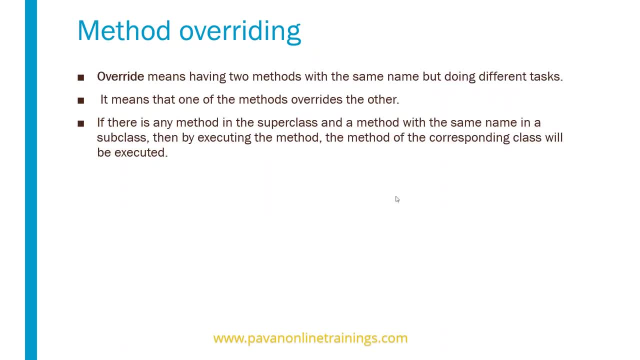 So this polymorphism can be achieved by using overriding and overloading concepts in Python. Now let us see What is method overriding first. so method overriding means Overriding can be applied for methods as well as variables. We can overwrite the methods and also we can overwrite the variables. 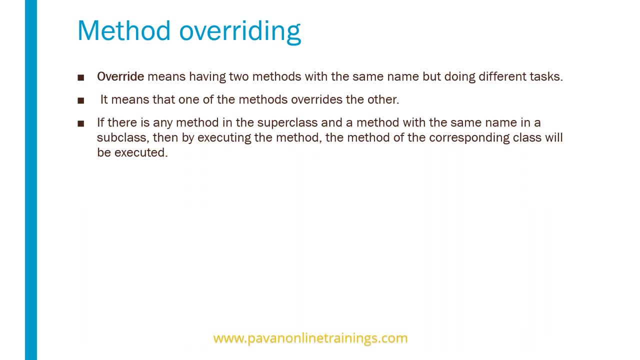 So over. it basically means having two methods with the same name but doing different tasks, Having two methods with the same name but different tasks, and it means that one of the method overrides the other. Okay, So, for example- let me just give you an example- 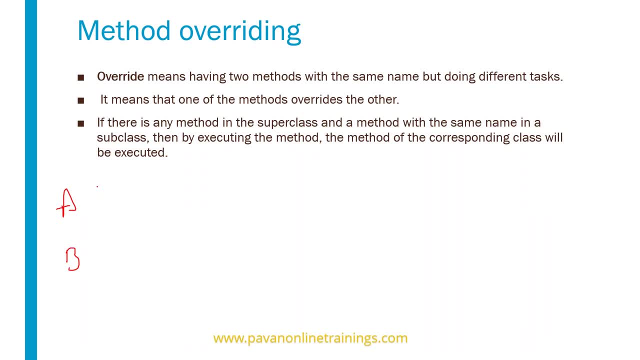 So, for example, I have a class a and also class B. So in in class a I have defined one method called as a. for example, let's create a display method, Right, and the same method I have again created in class B, Right. So on, the a is extended into class B. Now B is a J class of a. now, when they create the same method, 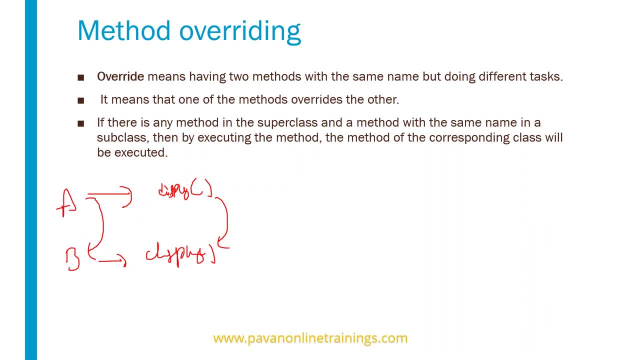 In class B. So what we are doing here is we are overriding this method. So when I create an object for class B, That will execute the method which is created inside the class B, And when I call this method from class a, and it will execute this from class. 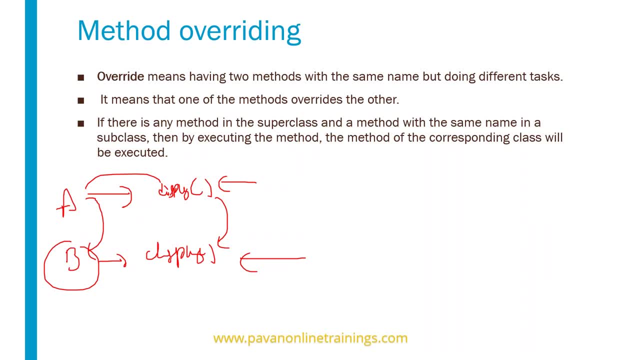 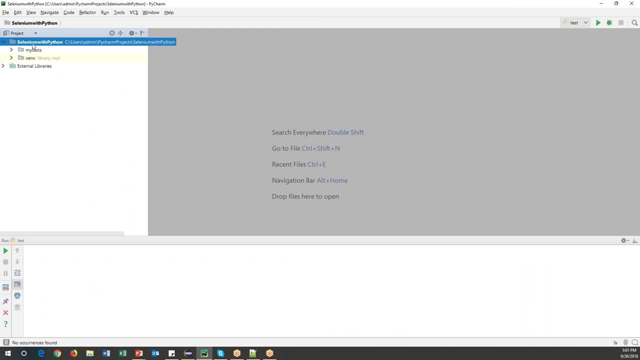 Okay, so this is called method overriding. now Let us see few examples on method overriding concepts. practically So let me open the pie channel. So here I am going to create a new Python file. I will name it as a polymorphism, Polymorphism test and. 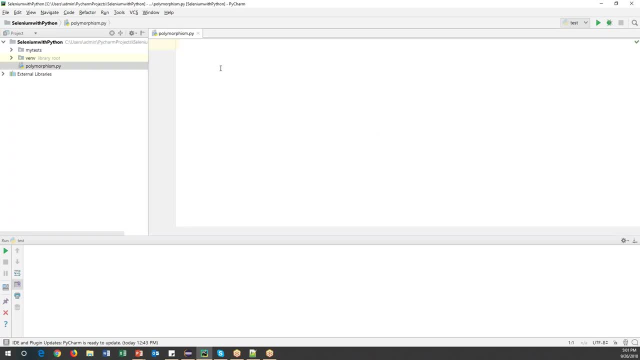 Click on OK. Now what I can do is simply I will just try to overwrite the variable. So overwriting concept can be used for variables as well as method. So in this example, I am going to show you how to override a variable. how to override a variable. 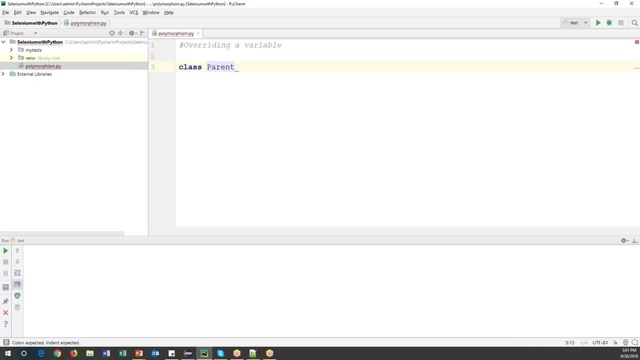 So what I can do is first I will create one parent class- Okay, parent. and inside this class, I will create a variable called name is equal to something called as a spot. Okay, this is a simple class which contains a variable. now I will create one more class. 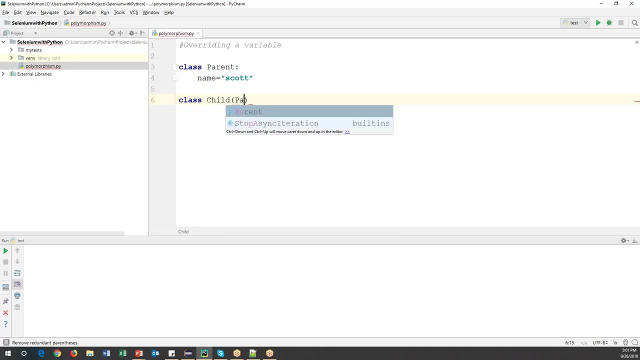 And I will name it as a child class. and this class is extended from parent class. This class is extended from parent class. now again, one more time. I will get the same variable here. I will just say, but this time I will code the different name, right? So this is a change. 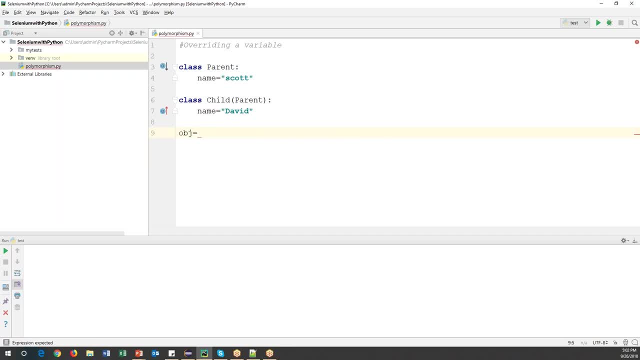 Now I will create an object for Change class. Let's say change, Right. So now what happens is when I call OBJ dot name, right, when I get a OBJ dot name and access and it's being this: well, you print OBJ dot name. So what this will print here we have just created an object variable for change last night 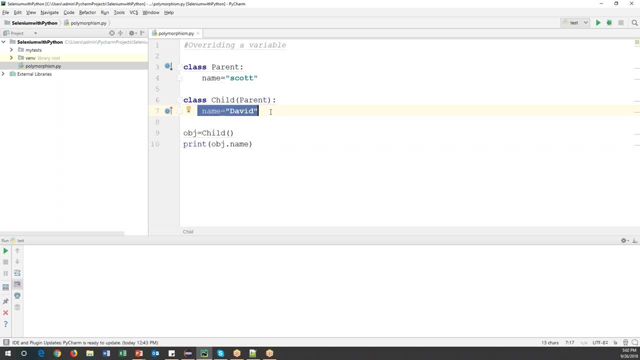 so change last, we already have the name is equal to David. so So even though the chain class, the standard, the fading class, the current and the latest value of name variable is dividend, So this should ring David, So it should think David. now let's run this code. 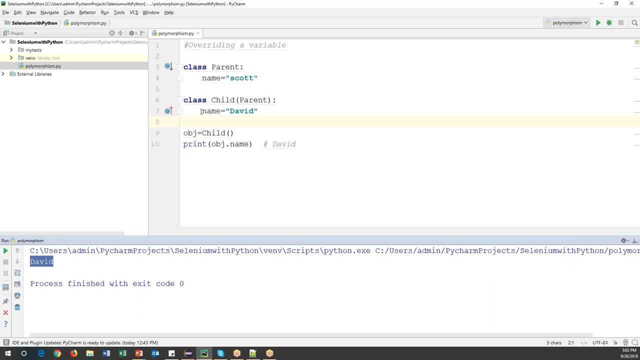 Now you will get. the baby doesn't on good. so that means the latest value, whichever we have overridden, so that value will be printed. so, for example, in the change class i haven't implemented anything, i'll just say pass and which variable it will call now. so 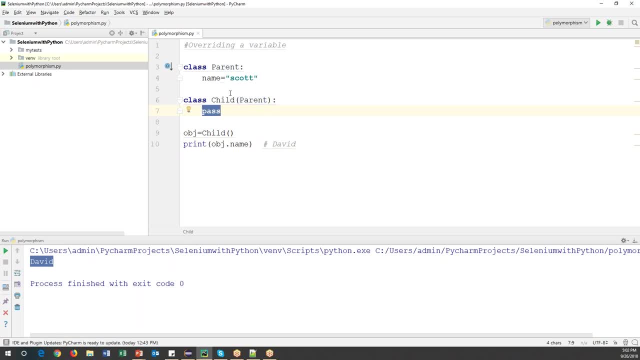 first it will go and verify the change class. so it doesn't have anything. so obviously it will execute or it will call the parent class variable. now when i run this, it will give you pairing class right. so this is small concept of overriding a variable. overriding a variable. 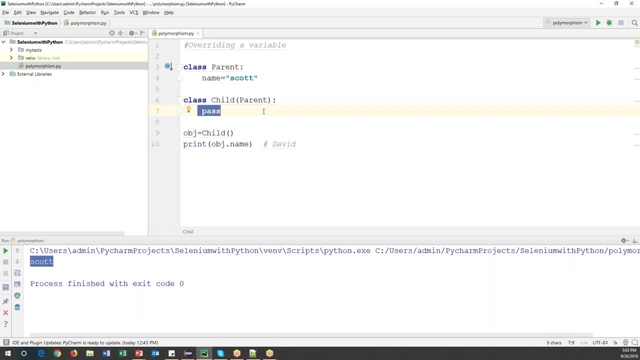 now i will also show you how to overwrite the methods. how to overwrite the methods? now let's go to with another example. so in this example i am going to show you how to overwrite the methods. so let's say again: here i have a class. i will define a class called as a. 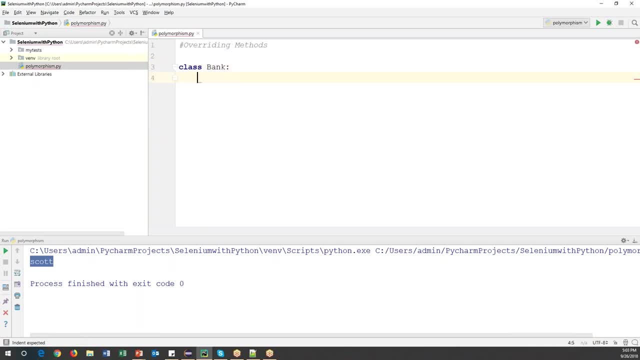 bank. okay, so this is my bank class and in this bank class i will create a method. let's say: rate of interest, rate of interest. so this is a method i have created, so this is a method, right, right? so inside this method, i will just return some value. let's say: 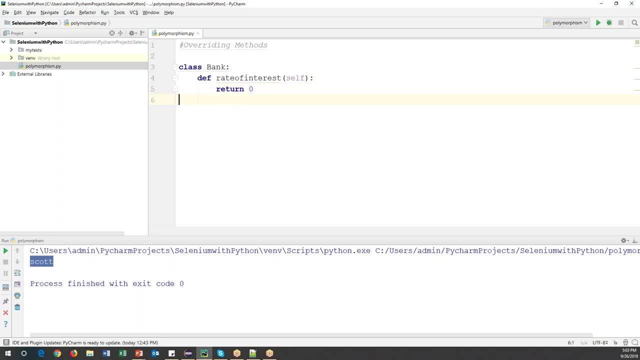 i'll return zero right. so, similarly, i will also create one more class and let's say icici and this: this particular class is extended from a bank class. this class is extended from bank class. now what i will do is, in this icsa bank, i will overwrite the whatever method we created in the 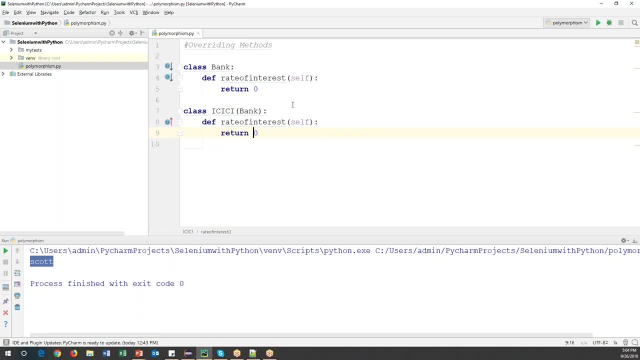 parent class. let me overwrite this now. here the rate of interest will be different. let's say 10.5. so now what i have done is i have just created one more shell class of the bank and i have just overriding the same method. overriding the same method. now, if you see this, in two classes, same. 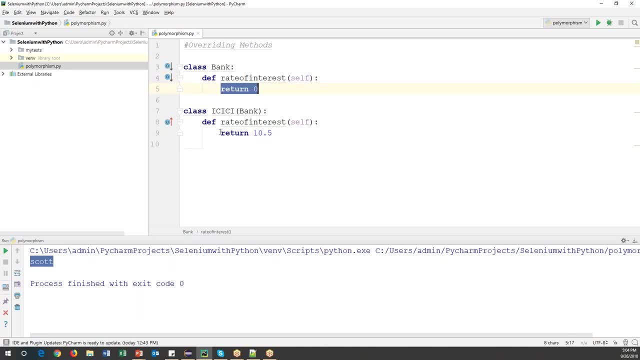 method we have, but it will perform different jobs. so here it will return zero, here it will return 10.5. same thing and two different functionalities, right? so this is a polymer visit. so let's say I have just created one object, right? So if I create an object for this class, 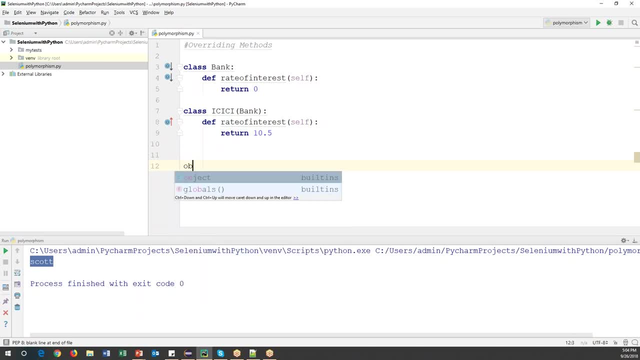 let me just create an object. Let's say OBJ- okay, is equal to. I'm just creating an object for ICICI. Now, using this OBJ, when I call a rate of interest method, So what this will execute now, so it will not just recall this method. 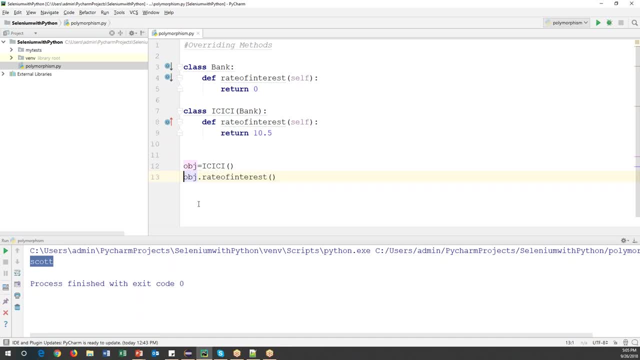 it just return the value. it will not print anything, right? We have to print that return value, So we have to use print function print method here. So now what happens? I have just created an object for ICICI, which is a child class. 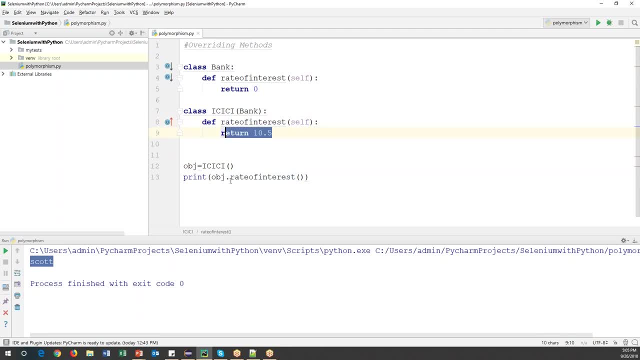 Now I immediately calling rate of interest method, So it will return 10.5, and here 10.5 will be written. Now, when I run this, it will give you 10.5.. So what does what we have understood based on this is: 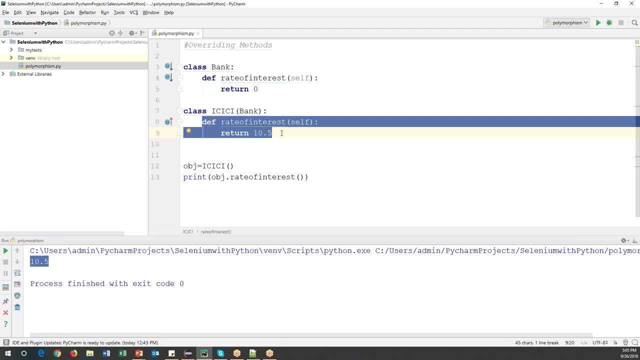 we have just over it in the method. As soon as we over it in the method in the child class, we, whenever we call this class or whenever we create an object for the child class, it will call the latest method. okay. 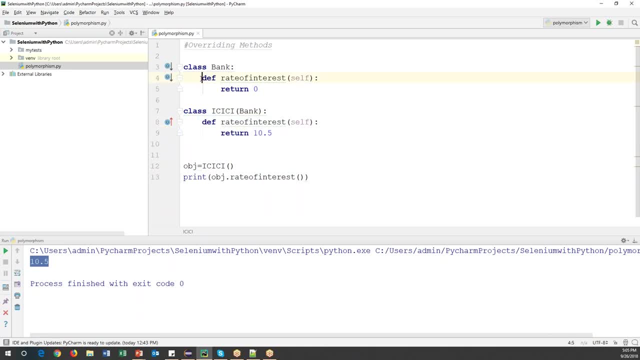 If sometimes, if the latest method is not available, then it will go up and call the pairing class method. okay, If this class is. if this method is not available, then it will go and call the pairing class method. It will go and call the pairing class method, okay. 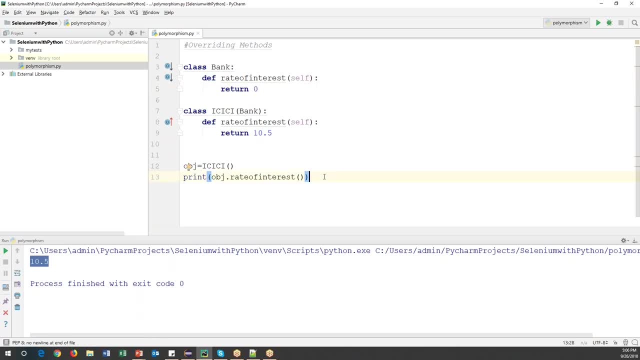 So, for example, if I want to call specially pairing class method, I have to create an object for bank class. Let's say one more object I'm creating OBJ. one is equal to bank, And now you can call this bank class, let's say bank. 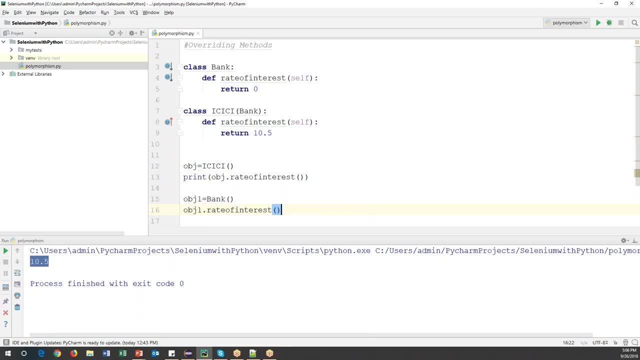 and OBJ one dot rate of interest. So when I call this now, it will call the method from the bank class. Now, when I run this, it will give you 10.5.. Okay, so this is again called as an overriding concept. 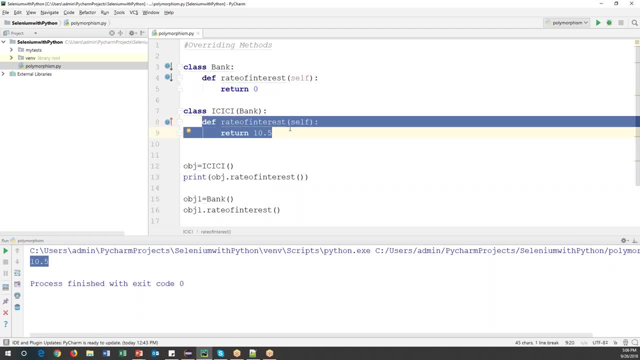 Same method we have used Again, we have overridden in the child class. We can create any number of child classes like this, And one thing is performing many forms. So one thing, the same method is performing multiple jobs, Right. so this is a kind of overriding concept. 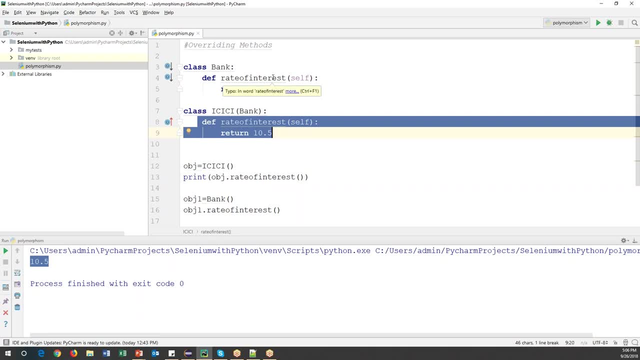 So we have seen overriding of variable and also overriding of methods. Overriding means same thing, same method will recreate in the child class. That is called as an overriding concept. So with overriding we can also achieve the polymorphism. And there is one more concept called as a overloading. 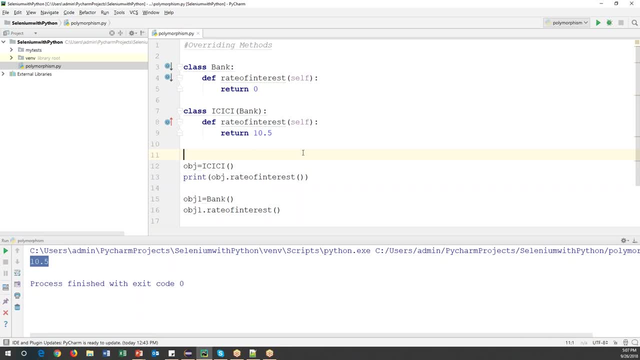 Overloading. So by using overloading also we can achieve the polymorphism concept in hoops, object-oriented. Now I'll show you how to work with the overloading, And before that let us see what is overloading. So in Python you can define a method in such a way: 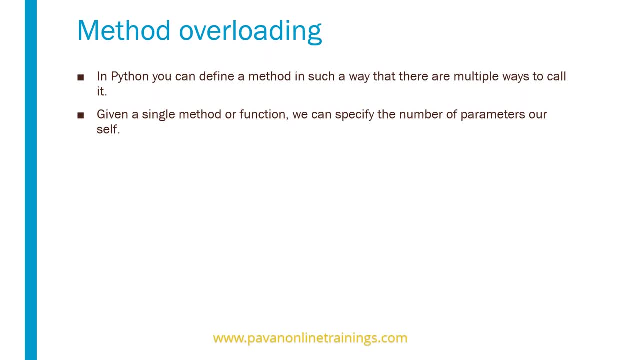 that there are multiple ways to call it. And, given a single method or function, we can specify the number of parameters or self Okay. so let me just give you one example. So, for example, if I create okay, so, for example, if I create a method, 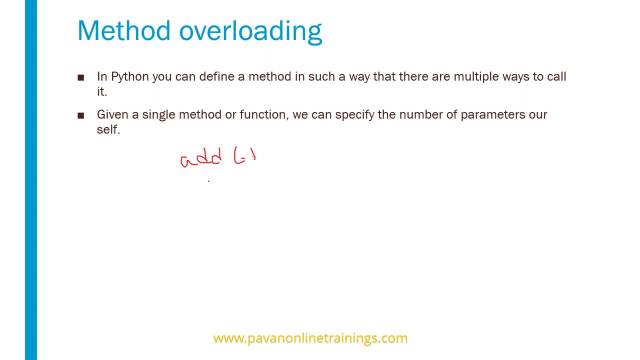 let's say I have created add method And here we need to pass some parameters. So based upon the number of parameters it will execute on specific methods. Suppose it is taking one comma two, the other method is taking. so suppose if I pass one comma two. 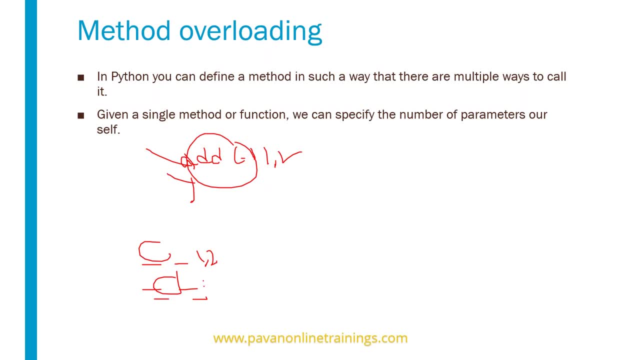 the same method will do, will act something different. And if I pass different parameters and the same method will be called and it will act it differently. And if I pass different parameters again, it will act again differently. Same thing will be differently behaved. 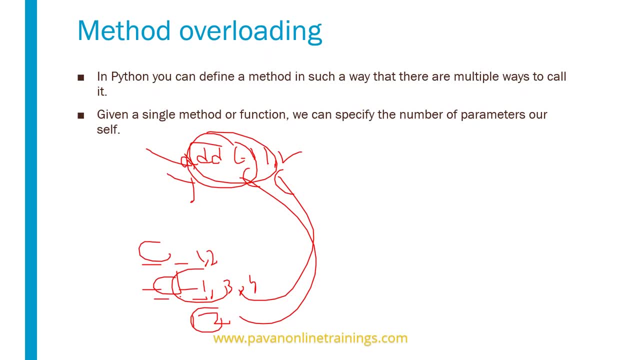 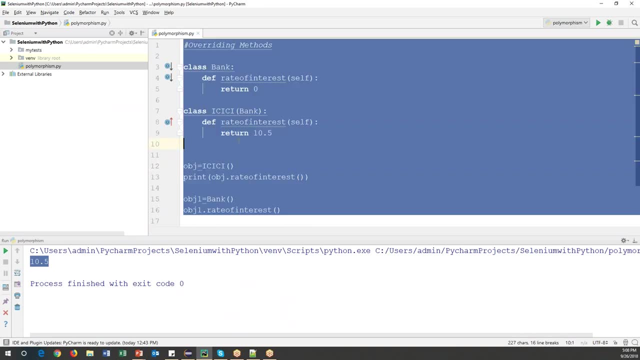 based upon the inputs we provided. Okay, this is a kind of overloading concept in Python. Let's see a few examples on this. Let's go to Python one more time. I'm removing this, So here I'm going to show you one example for overloading. 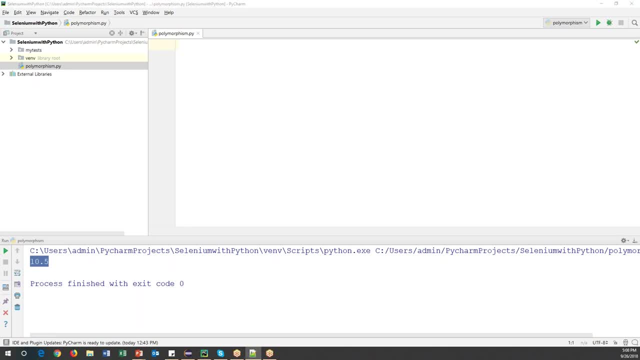 how to overload methods. how to overload methods? So to demonstrate this, what I can do is I will just create one simple class called as a human right. So in this class, I will create a method called diff Say hello method- say hello method. 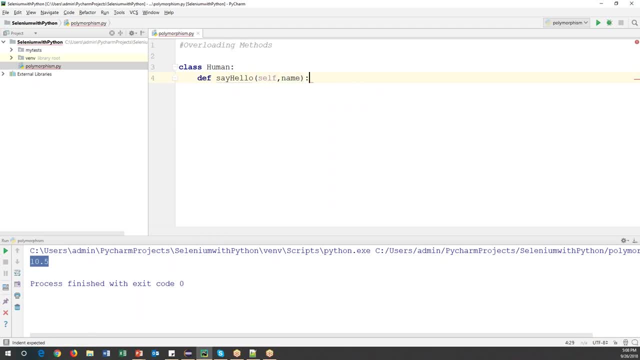 And here I will just pass one parameter called as a name. All right now, here, what I can do is I will assign the default parameter is none, Suppose we can pass the value for the name from the actual method, Or if I don't pass anything, 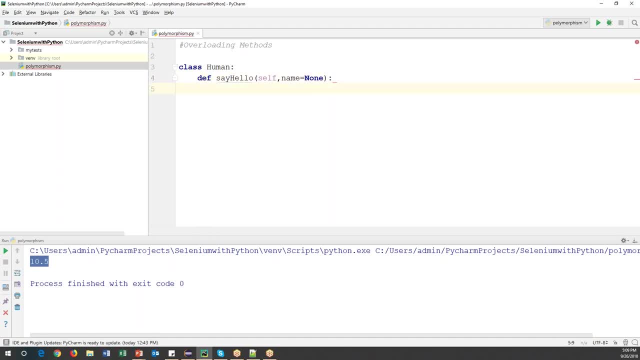 it will by default assign the none to this variable. Okay, now, in this method, I will just put one condition: If name is, if the name is not none, okay, if the name is not none. what I should do now is I should just print: 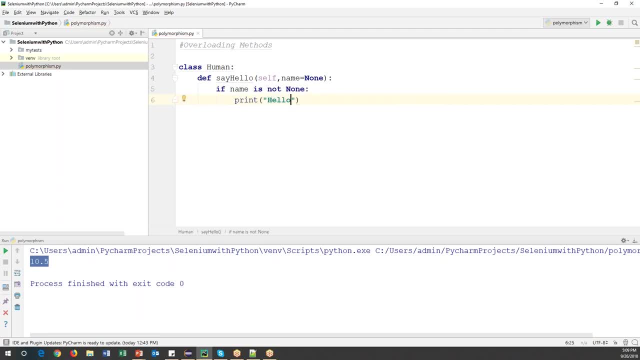 I should just print hello, hello, just print hello, So not none means it contains some name, right? So name is equal to none. I put: This is the default variable. Suppose if I pass some name, suppose if I pass some Scott, so name is equal to Scott. 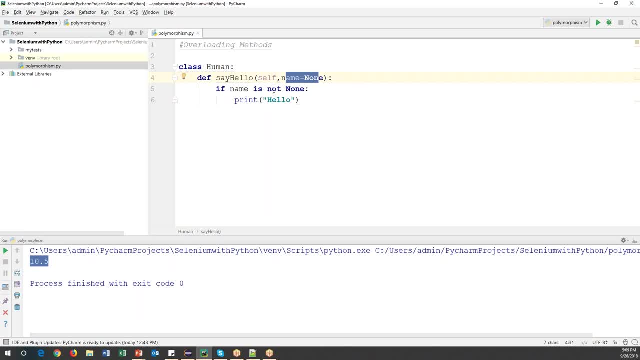 Now here, what I'm saying is: I'm checking the negative condition. If name is not none, that means there should be some name, right? So here, hello, I will also append something called name concatenate with the name. So the hello, concatenation with the name. 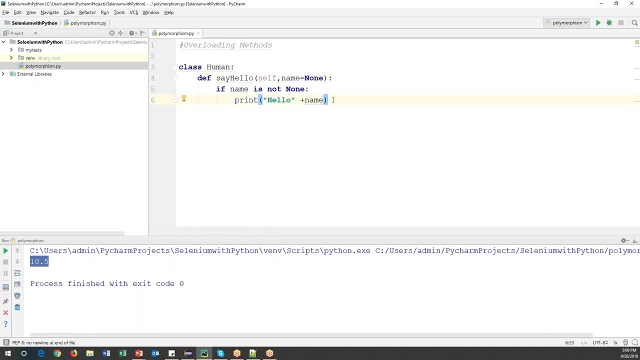 whichever we provided here. This is a one conditional Suppose. if I didn't pass any value for the name, that will be taken by default as a none right. So here in the else block, in the else block I will write print, just help. 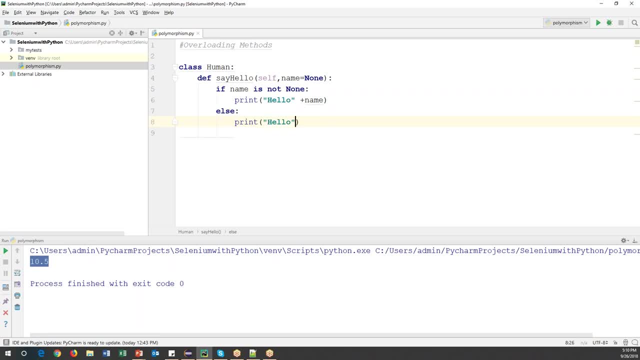 Okay, just hello Now how it will execute whenever I call this method, If I pass a name to that particular method. so the first condition will become true, So it will print a hello along with the name, Suppose if I don't pass anything to this particular method. 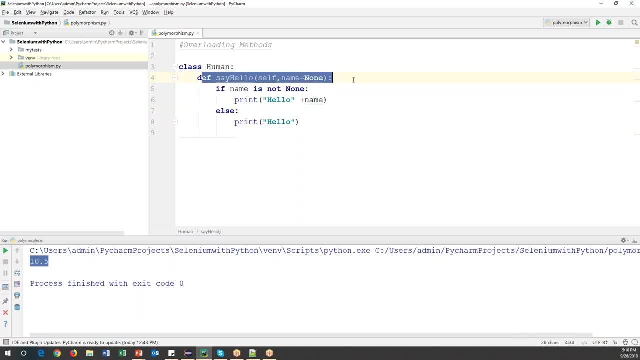 just it will execute L part. So the same method will behave in two different ways. We pass a name, it will behave differently If I pass. if I don't pass a name, then it will differently behave. So let us see how we can call this method. 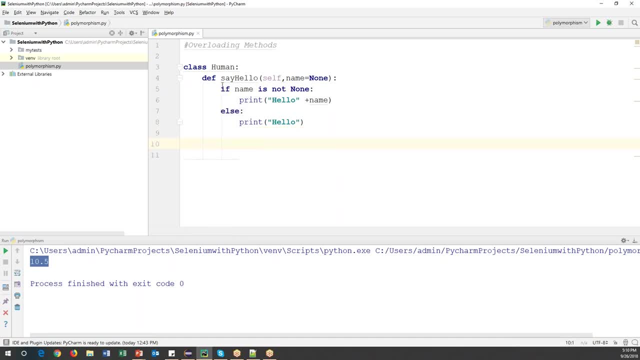 Now, this is a class which contains a method I created. Now, if I want to call this method what we can call, we can just need to create a object for human right. So let me create: OBJ is equal to human. 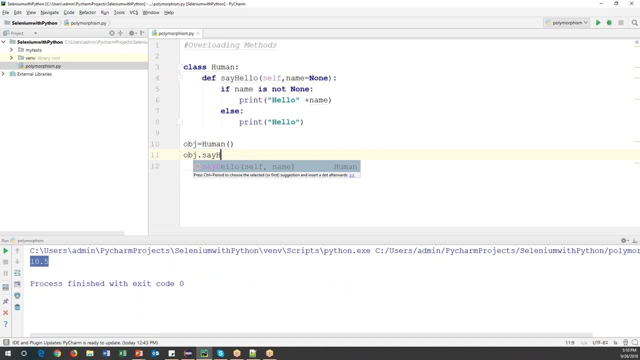 And by using this object I will just say hello. I'll just all say hello and observe this carefully. So this time I'm not passing any value. this time I'm not passing any value. So what happened now, when I don't pass any value by default? 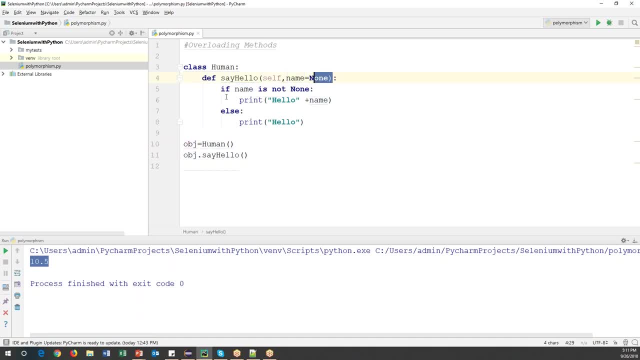 the name will be none. None means no value. So what is the condition now? if name is not none, that means name is none, means the else part will be executed here, because when this name is equal to none, if it doesn't pass anything, okay. 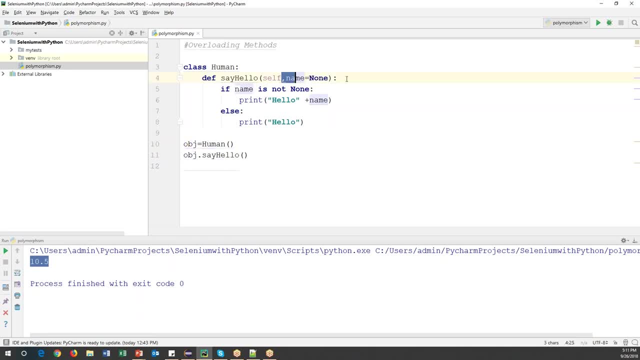 if I hear I'm not passing anything right. Anything means the name will be assigned to the none. So if a name is none- what happened now? it will execute only else block. If name is not none, then it will execute hello, along with the name. 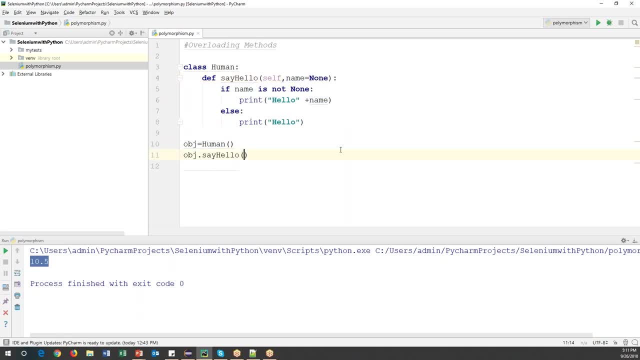 If the name is none, Okay. Okay, Let me just pass one variable here. Let me just say I'll pass my variable. I'll pass my name. observe this now. So I'm not passing the name. what happens now by default name values and none. 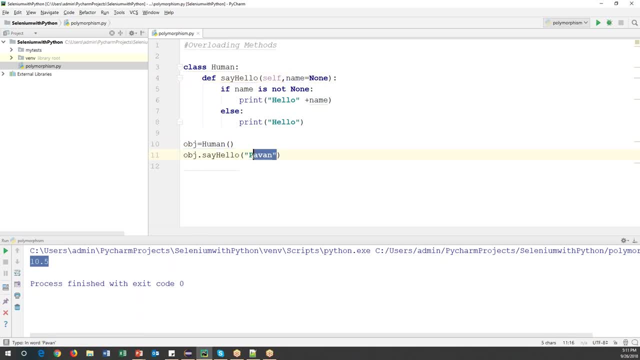 but if I pass some value, what happens now? name value becomes oven. So now what happens if name is not none? So the first condition, if condition will becomes true, if the name is not none because name value and passing it here, So name is not none now 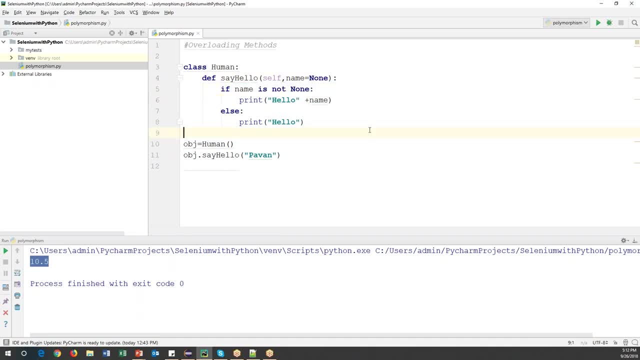 So then what happens? If the name is not none, it will print Hello name, right? So when I exclude this code, it will print hello power. All right, suppose. same method. I will call one more time, But this time I didn't pass any value here. 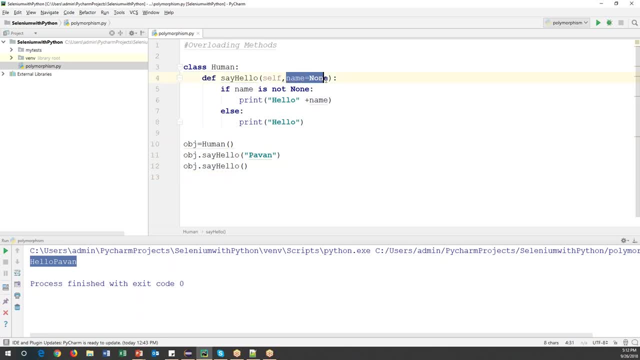 And then what happens? if I didn't pass any value name will be assigned to the none though name. then if condition will not match, when this? if condition will match. if the name is not none, then it will match, but here we are passing the empty right. 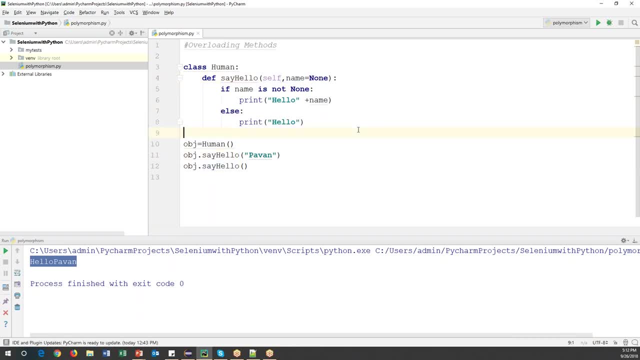 That means it is a none. none means else. blog will exclude now this time It will also give you only hello part. So what we understood based on this, the same method will behave in two different way. two different ways. If I pass parameter behaves differently if I didn't pass any parameter. 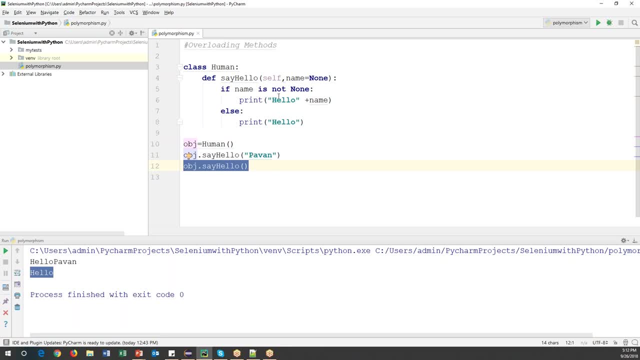 it different, behaves differently, right, So this is a kind of a polymer prism. cause the same thing and the behavior is different. All right, so this is a kind of polymer prism, All right. Now I'll show you one more example. 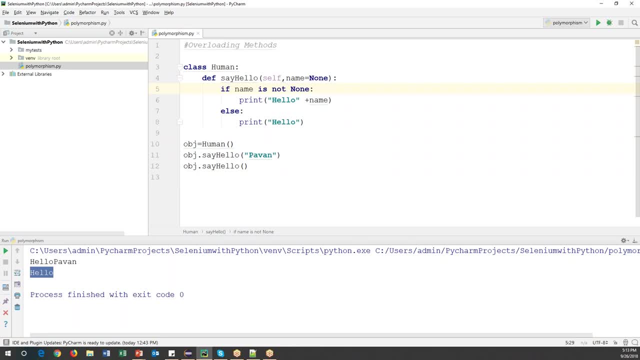 This is one example for overloading methods. Now I'll show you one more example for overloading methods, and here what we have done is okay, So let me just show you again. This is again example for overloading methods. overloading methods. 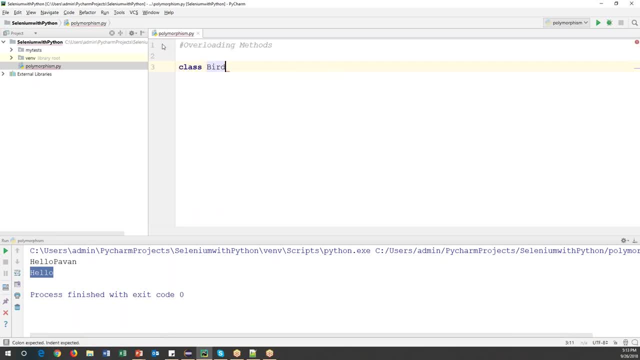 See now, what I can do is I will just create one class called as a bird, and in this class I will create a function Method, that's a def live method. and here again I'll do the same So self and I'll just say I'll pass a bird name here later. for now, 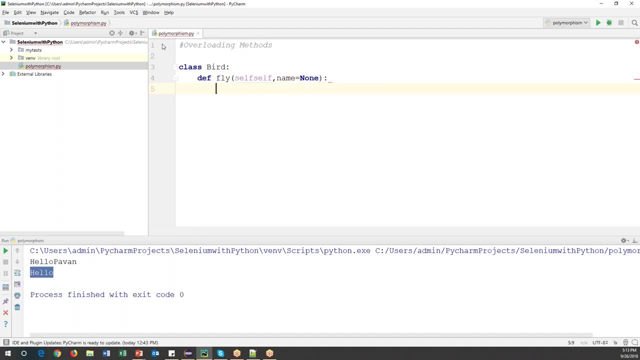 I'm just making as a nun. Okay, here I will create one condition: If, if name is equal to name is equal to right. Let's say, parent name is equal to parent. If the bird name is equal to parrot. what I should do, 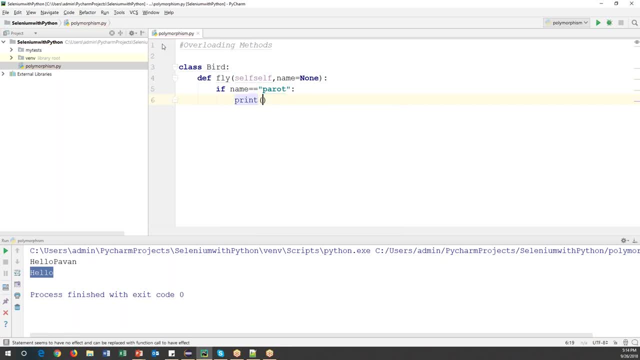 Now I will just print here. Okay, I will just print here. So parrot cannot fire, can flying, so parrot can fly, right, So I just say: can fly. Okay, Suppose, if this condition is false, let's write one more condition. 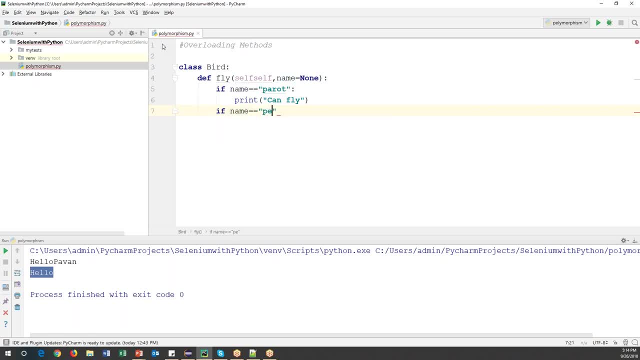 If suppose name is equal to, let's say, penguin, Okay, suppose name is equal to penguin. So now what happens? expelling is wrong, right? G U I N right. So if the name is penguin, this is also bird. 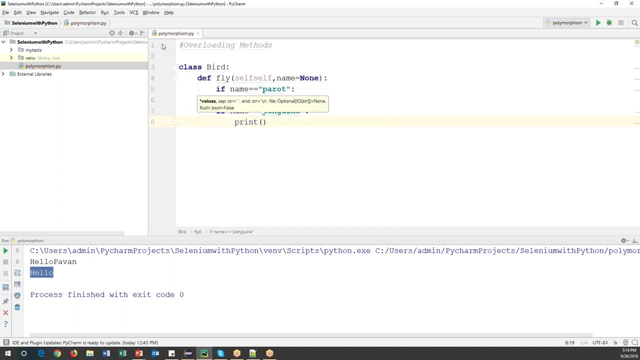 So if the name is penguin, it cannot fly, right, So I'll just say cannot fly. Okay, Now I had two different methods. I already suppose if, if name is none. So suppose if I didn't pass any name for the bird. 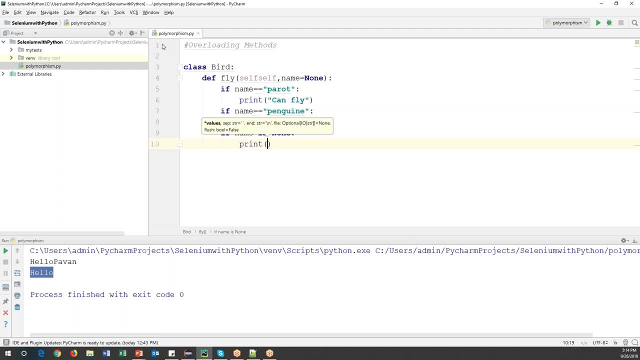 what should execute. it should execute. no input, It should execute. I'll just say: no input, no input. So I have just created a method inside The class- the method name is flying- which will take one parameter name as a parameter if the name is a parrot. 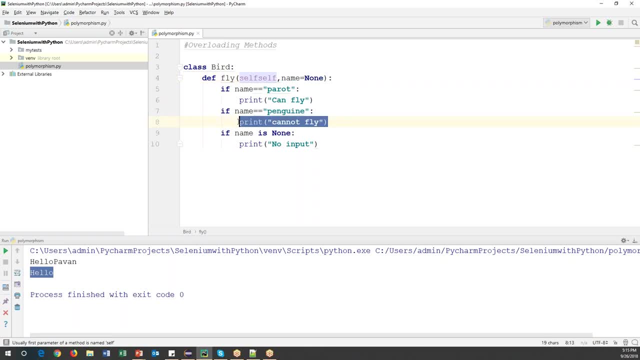 then it will print: can fly if the name is a penguin. It cannot fly if the name is none. means if I didn't pass any bird name, then finally the last one will be executed right. So the same thing, same fly method, and I will pass different kinds of inputs. 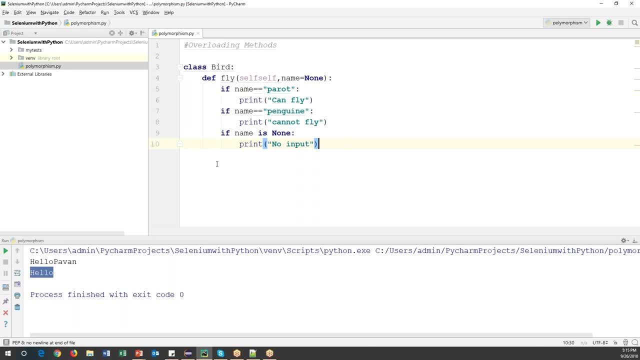 and different kinds of output we will get. now here I will just how we can call this method through this class name. So I will just create a object for this bird class, right. So now, using this object, I will just call fly method or fly function. 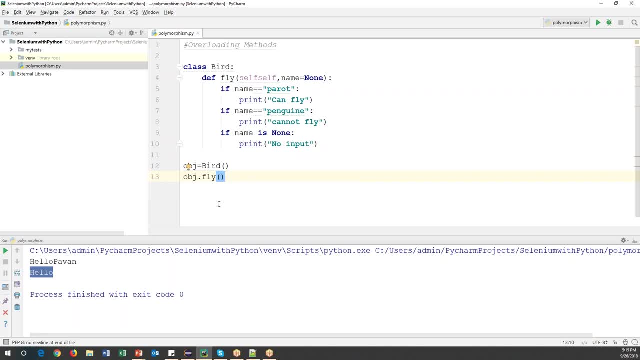 Go see first time. I'm not passing any parameter. Now what happens? so it will go here if I didn't pass any parameter, So name will be assigned to the none by default. none means, if the name is done, what should happen. no input is provided. 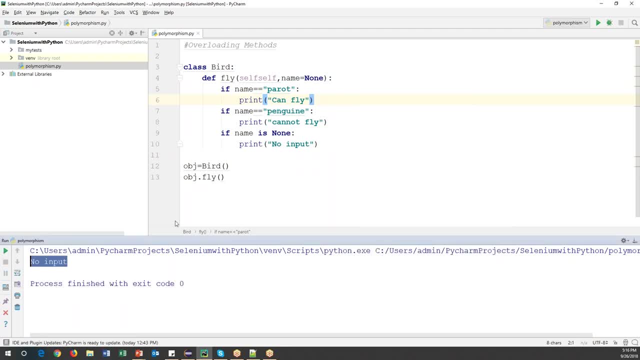 So when I run this code, no input. is there no input? and suppose, suppose, if I pass something called as a parent, let's see Parrot. now what happens? the name will be assigned to the parrot, The first condition will becomes true and it should. print can fly. 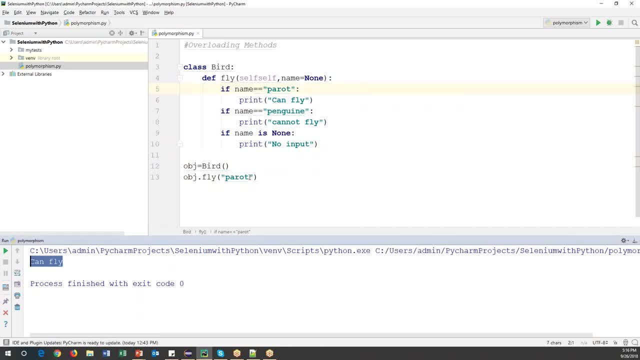 Now, let's run this. it should. print can fly. So same method and calling by passing different kinds of inputs or parameters and behavior will be different. Now, instead of this, I will pass a penguin. I'll pass a penguin. now, when I run this, it will give: you cannot fly.